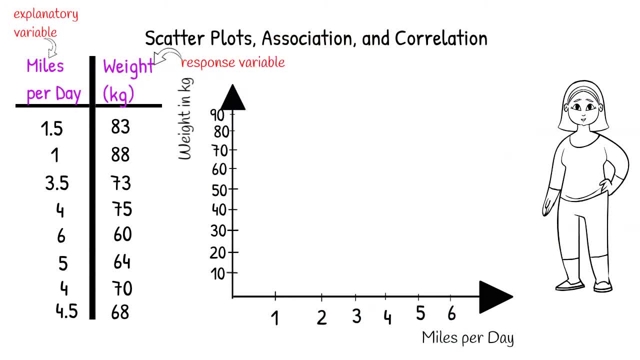 we go up to 90.. Our first point is 1.5 on the x-axis and 83 on the y-axis, Then 1, 88. Then 3.5, 73. Followed by 4, 75,, 6,, 60,, 5, 64,. 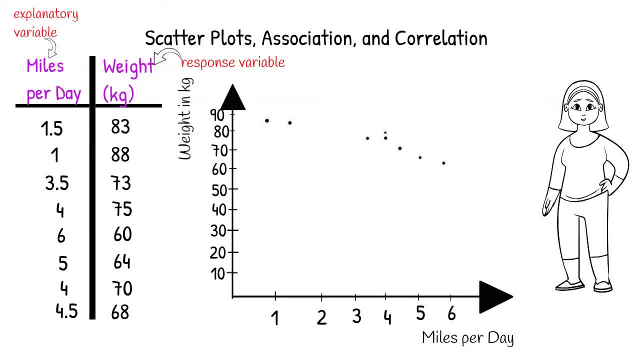 6,, 70, and finally, 4.5,, 68.. Notice that the points cluster somewhat in the shape of a line. This means that the number of miles walked per day is in some way associated with the weight of a woman. 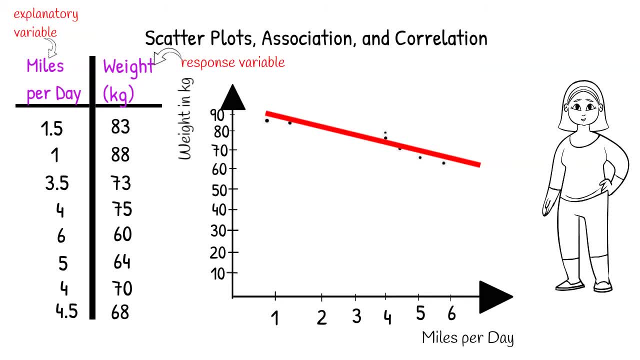 It is important to note, though, that though we may identify a correlation in our graph, correlation doesn't necessarily mean causation- In this example it might, since higher mileage does lead to more calories burned. but suppose instead our variables were number of dogs seen. 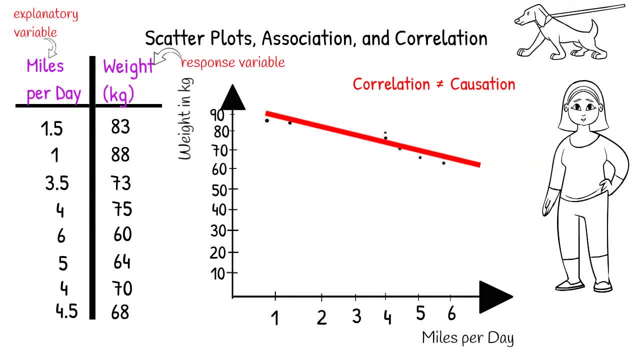 on the street versus weight. There might be an association between the variables, since the women were likely to see more dogs if they walked for longer. but certainly seeing more dogs on the street does not cause a person to be lighter or heavier. It is important when analyzing correlation. 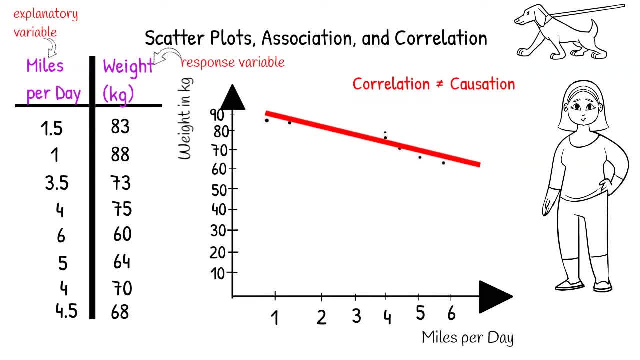 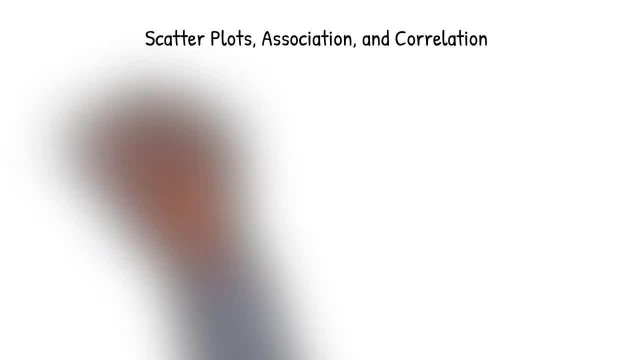 that we don't fall into the trap of assuming that correlation is the same as causation. Let's look more closely at the types of correlation we will come across. If our points take the shape of a line and have a negative slope, as x increases, y decreases, we say that there is a negative linear correlation. 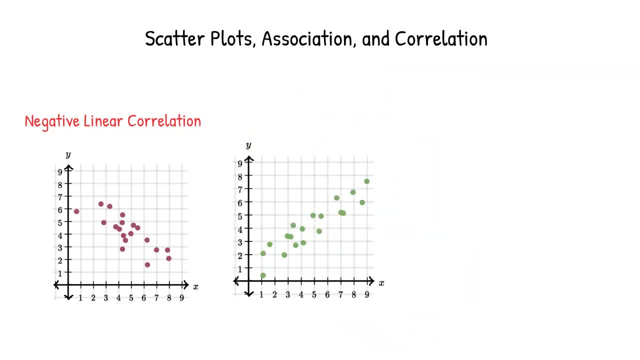 If our points take the shape of a line and have a positive slope, as x increases, y also increases, we say that there is a positive linear correlation. If we cannot identify a trend from a point, we say that there is no correlation. We can get more specific by also discussing the strength of 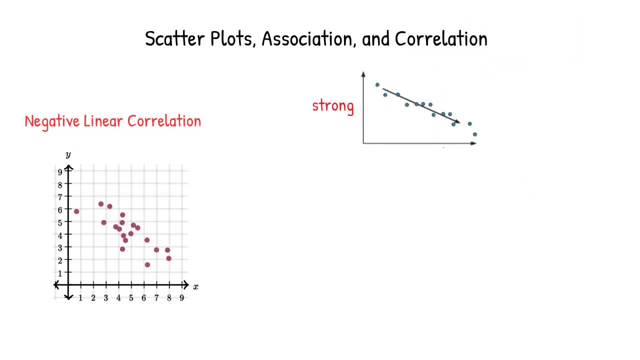 the correlation. There is a strong correlation if the points are clustered close to the shape of the line, a moderate correlation if the points are a bit more spread out, and a weak correlation if we can identify the shape of the line but the points are not clustered closely to it.